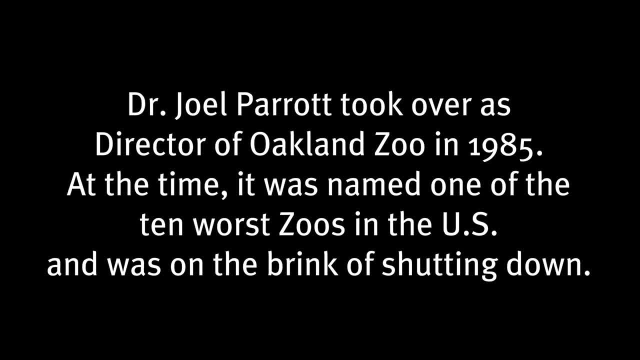 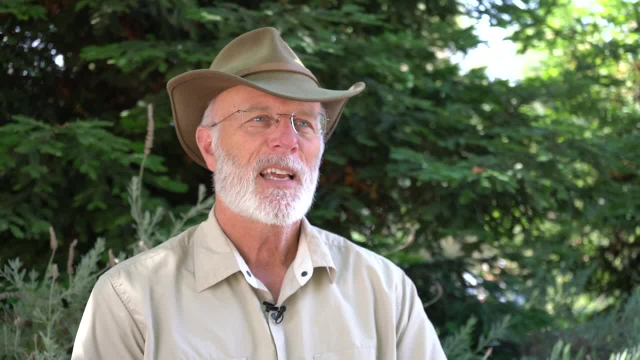 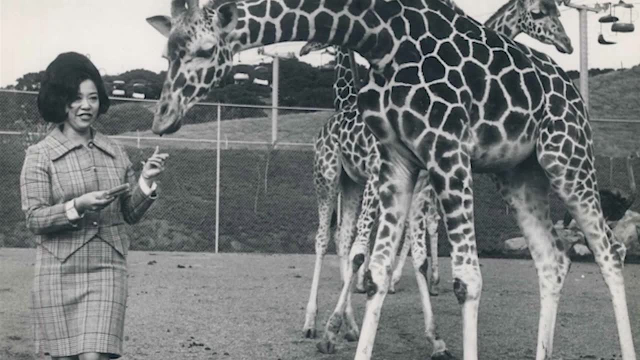 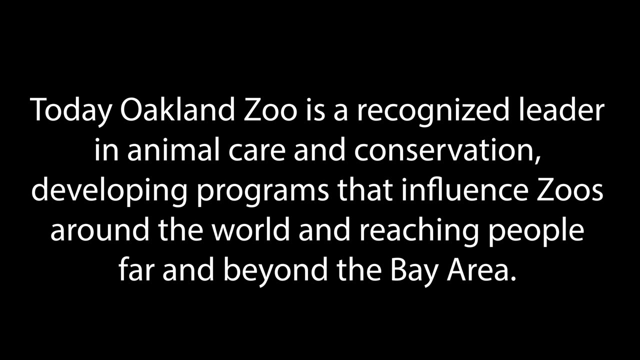 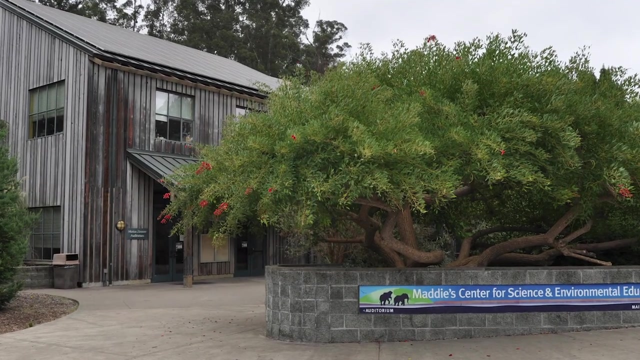 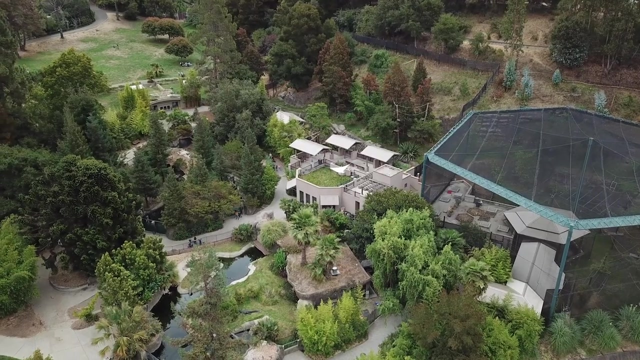 Back in the early days the zoo was a little rough. It had a problem with funding. A lot of the exhibits were just out of date, The major projects being our front entrance renovation, an education facility, a veterinary hospital, the elephant exhibit and the children's. 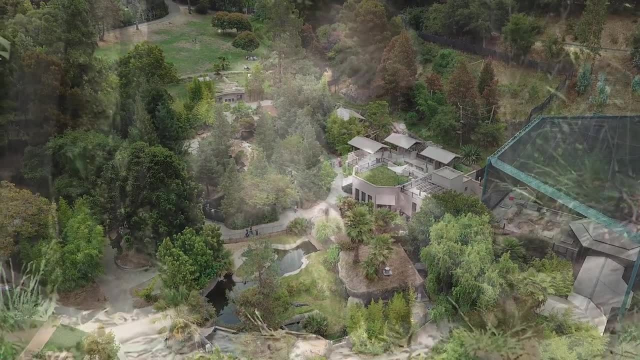 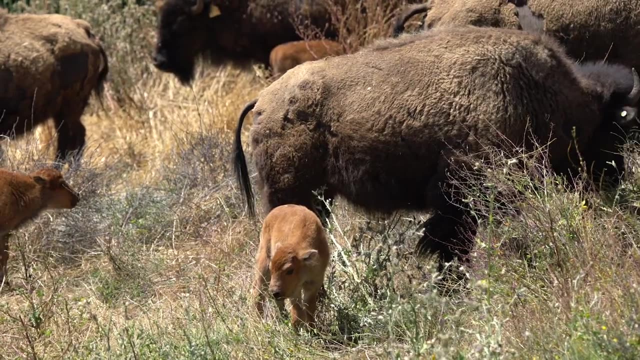 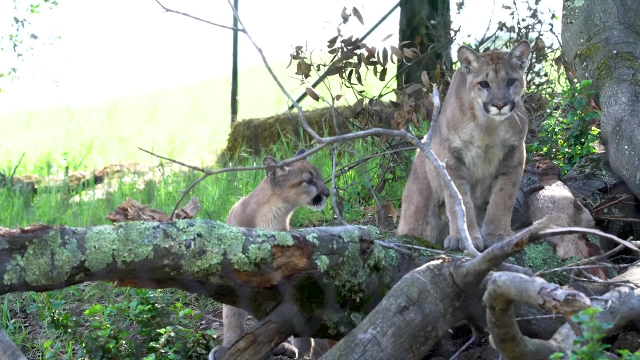 zoo. Once we really had gone through all that, we were able to say that we've renovated pretty much the whole zoo and we were ready to expand. Within that came the idea to why don't we focus part of the zoo on California's wildlife? That was the beginning of the thought about the California 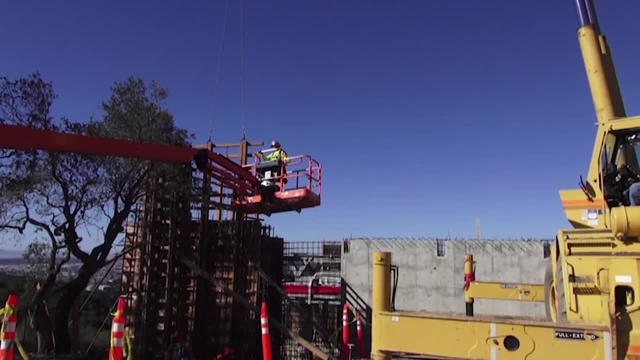 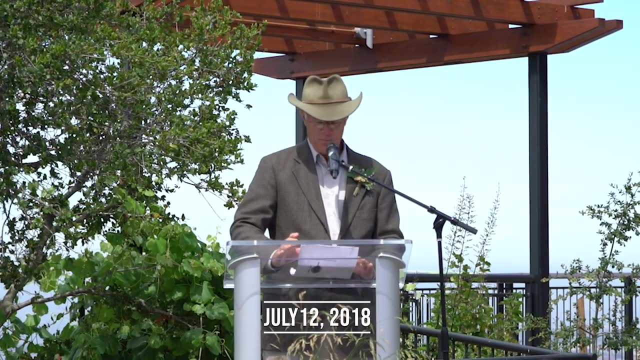 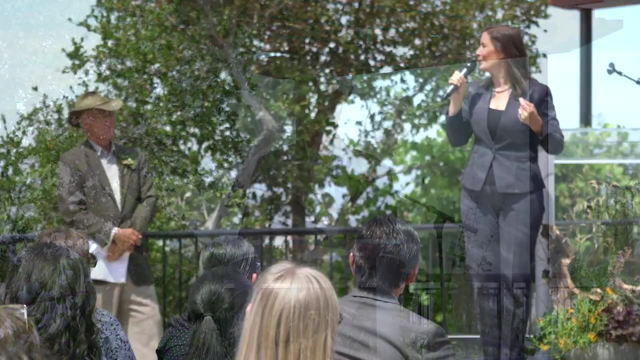 Trail. It's been a fun project because I've certainly learned a lot and I've sworn that this is going to be the last gondola I ever build, But I would like to welcome you all to the opening of the California Trail. This is not just an amazing project, an amazing gift for our current generations and our future. 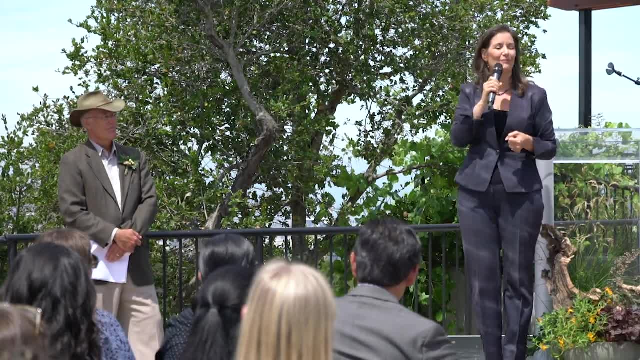 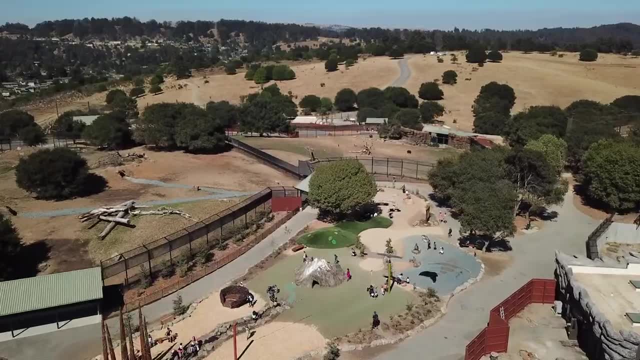 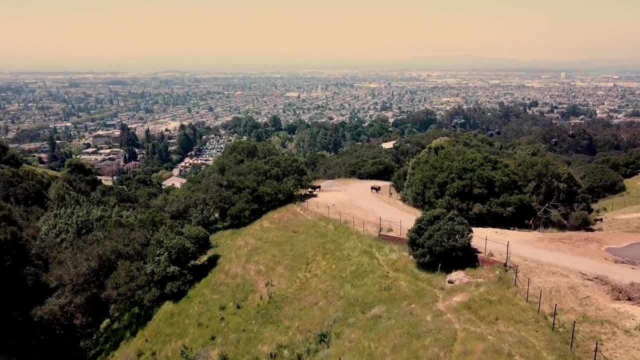 generations, but a bold expression of Oakland. It felt great to finally reach the end of the world. This is a long time goal to have a wild animal park right in the middle of what you could look out on, a spectacular view that no other zoo in the United States has. 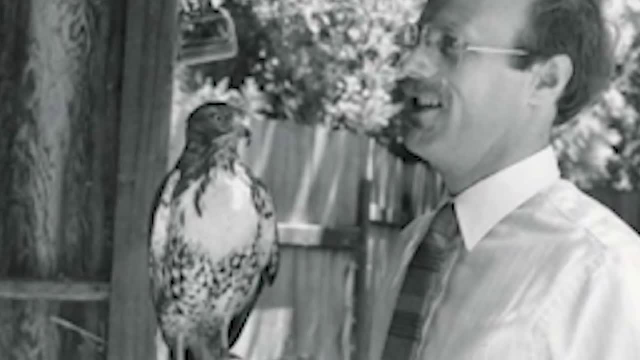 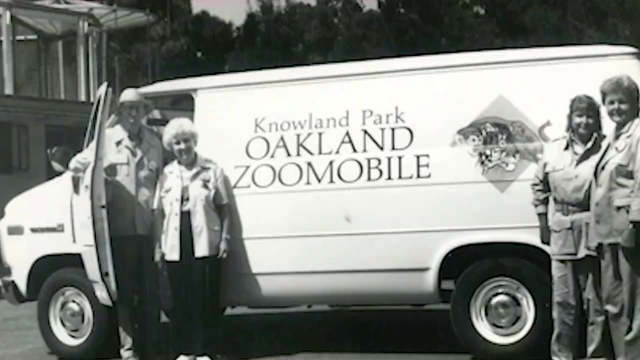 In the 35 years I've been here, the zoo has grown from attendance of about 240,000 to over 900,000. this year Our budget has grown from $2 million to $20 million. We've gone from a $25 million to a $200 million to a $100 million budget. this year We've been bringing 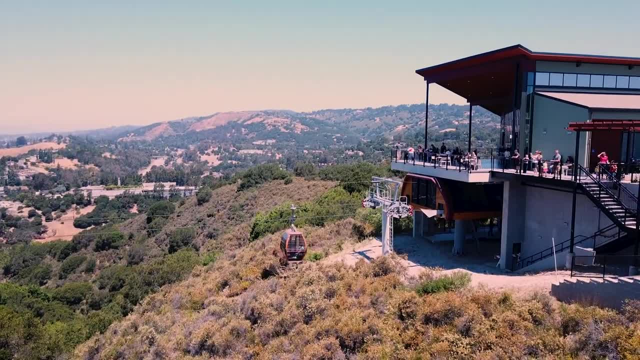 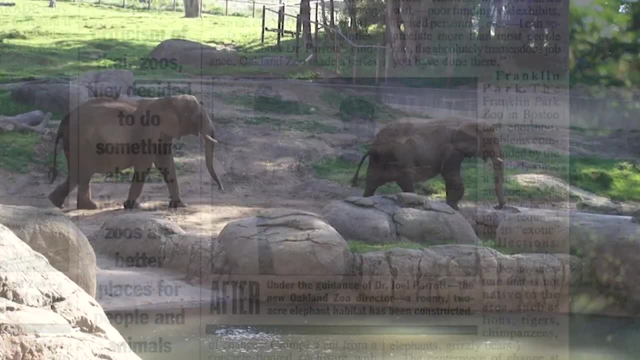 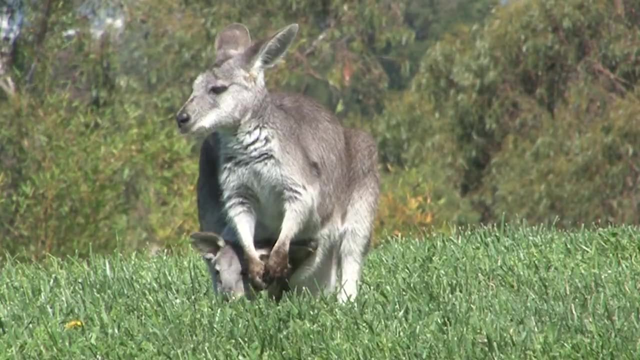 Zoo to now 100 acres, So it's just changed dramatically from what it used to be to what it is in 2018.. Every species we have here on exhibit we have a related field conservation project, because the world of zoos is more than 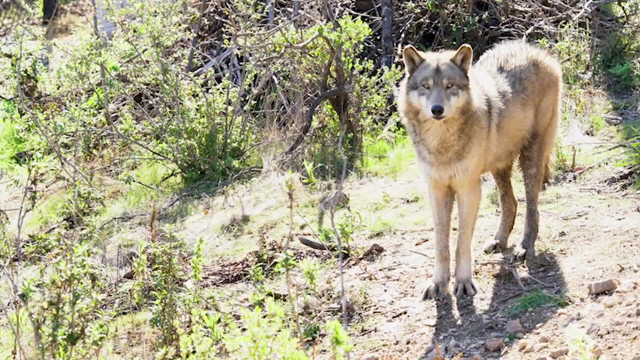 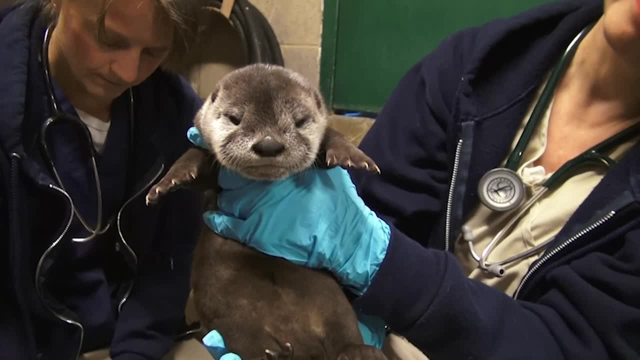 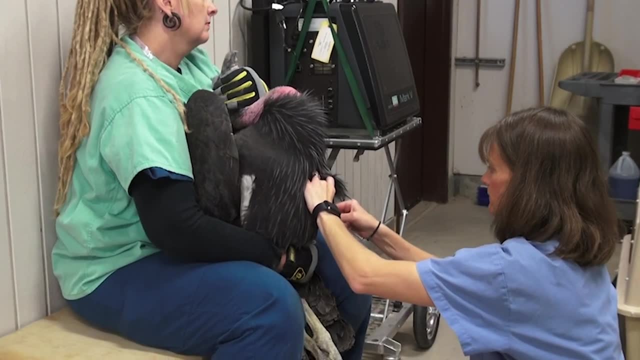 just one of the entertainment, and even more than education, The world of zoos is also about supporting wildlife in the wild. I think I'm most proud of the staff that has been built up that works here at the Oakland Zoo, because they put everything into it and they're just really good people. They care about their